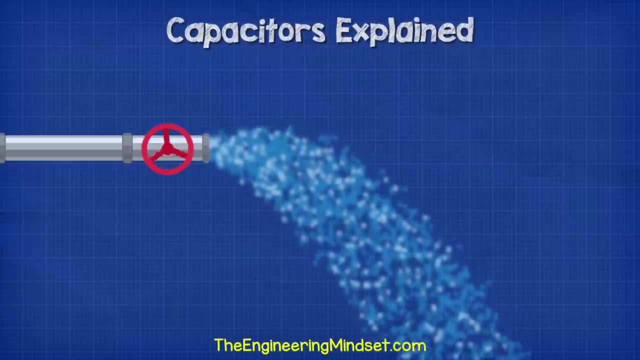 flowing through it. The water will continue to flow until we shut the water pipe. The water will continue to flow until we shut the water pipe. The water will continue to flow until we shut the valve. Then no water can flow. However, if, after the valve, we first let the water flow, 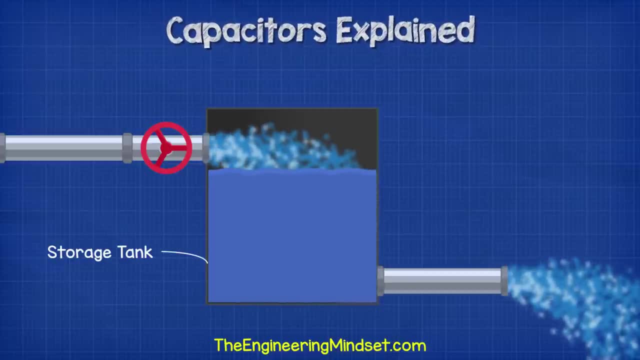 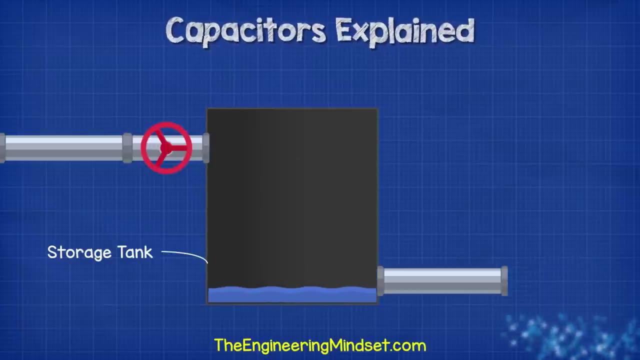 into a tank. then the tank will store some of the water, but we will continue to get water flowing out of the pipe. Now, when we close the valve, water will stop pouring into the tank, but we still get a steady supply of water out until the tank empties. Once the tank 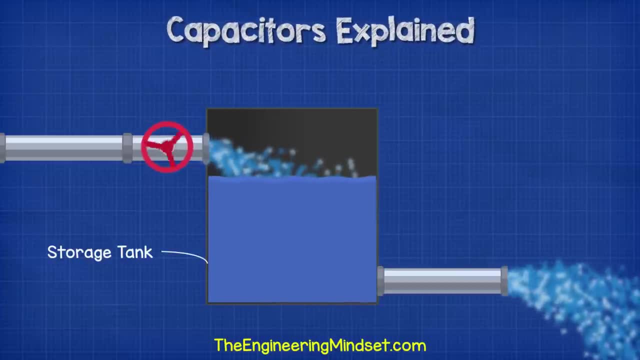 is filled again, we can open and close the valve as many times as we like. As long as we do not completely empty the tank, we will get an uninterrupted supply of water out of the end of the pipe. So we can use a water tank to store water and smooth out interruptions to the supply. 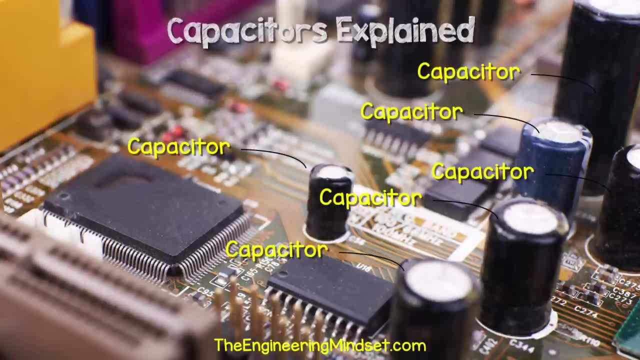 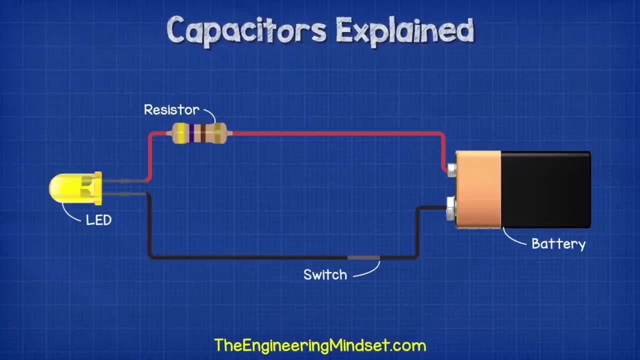 In electrical circuits the capacitor acts as the water tank and stores energy. It can release this to smooth out interruptions to the supply. If we turned a simple circuit on and off very fast without a capacitor, then the light will flash. But if we connect, 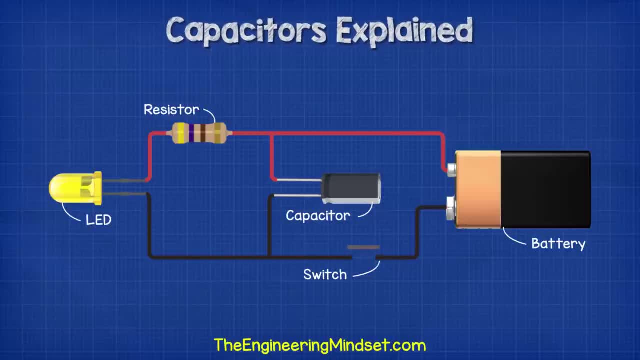 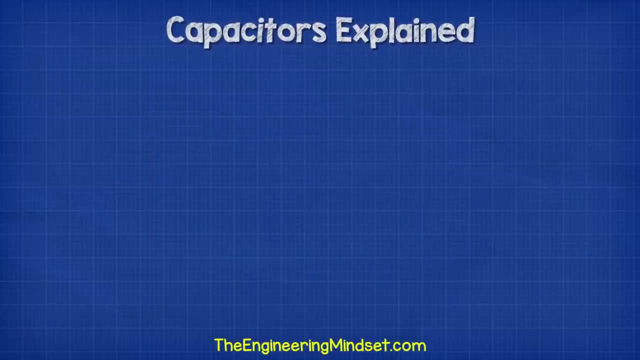 a capacitor into the circuit, then the light will remain on during the interruptions, at least for a short duration, because the capacitor is now discharging and powering the water. In a basic capacitor we have two conductive metal plates, which are typically made from. 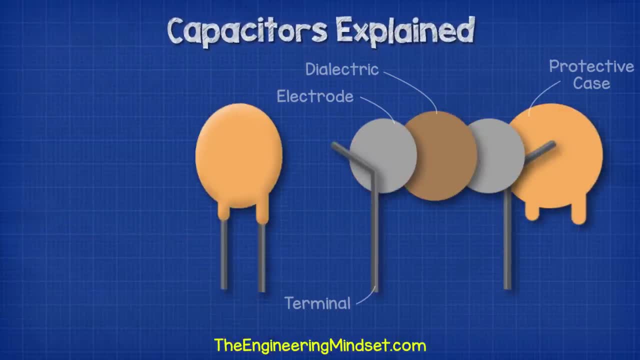 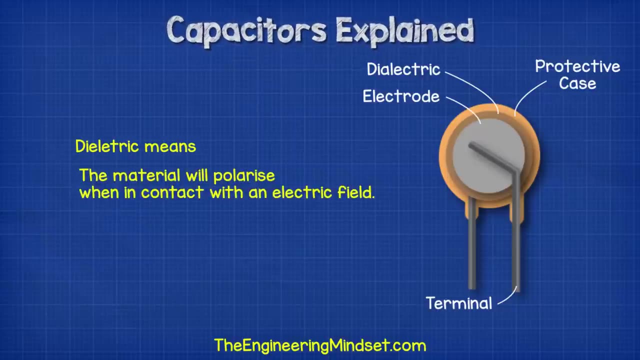 aluminium or aluminium, and these will be separated by a dielectric insulating material such as ceramic. Dielectric means the material will polarise when in contact with an electric field, and we'll see what that means shortly. One side of the capacitor is connected to. 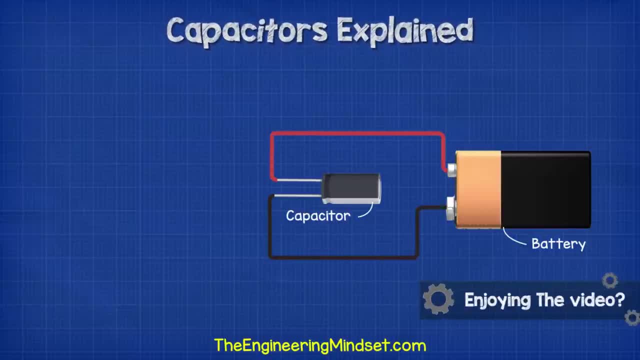 the positive side of the circuit and the other side is connected to the negative. On the side of the capacitor you will see a stripe and a symbol. This will indicate which side is the negative. If we were to connect a capacitor to a battery, the voltage will push the electrons from the 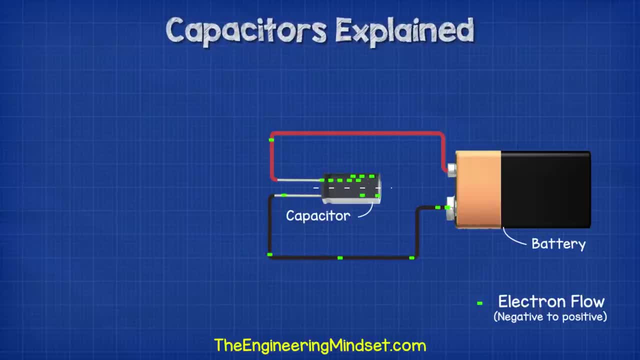 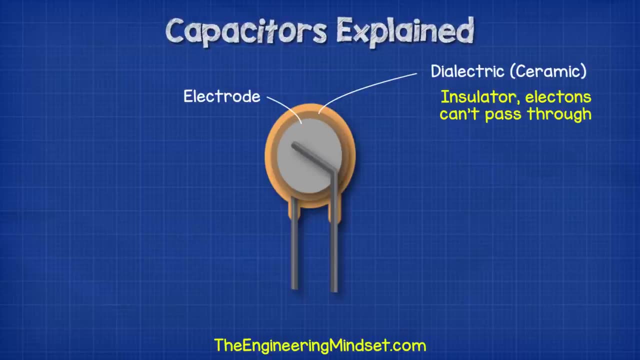 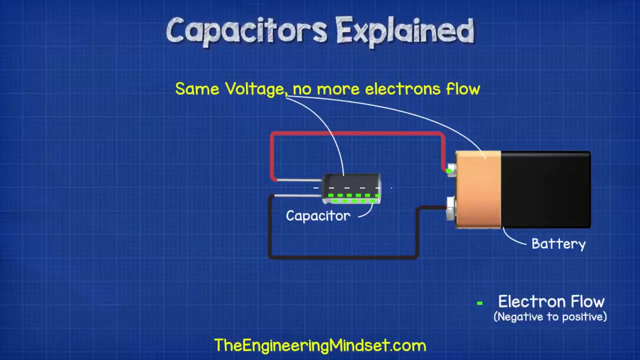 negative terminal over to the capacitor. The electrons will build up on one plate of the capacitor, while the other plate in turn releases some electrons. The electrons can't pass through the capacitor because of the insulating material. Eventually, the capacitor is the same voltage as the battery and no more electrons will flow. 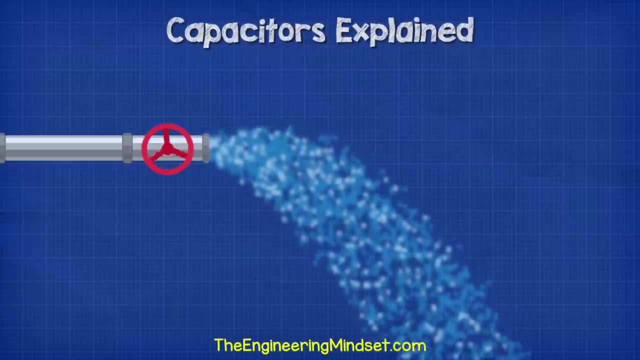 flowing through it. The water will continue to flow until we shut the water pipe. The water will continue to flow until we shut the water pipe. The water will continue to flow until we shut the valve. Then no water can flow. However, if, after the valve, we first let the water flow, 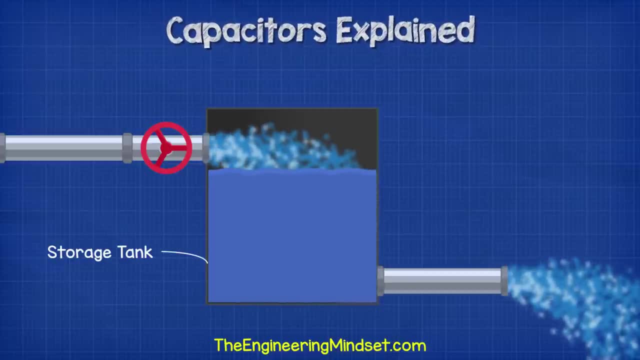 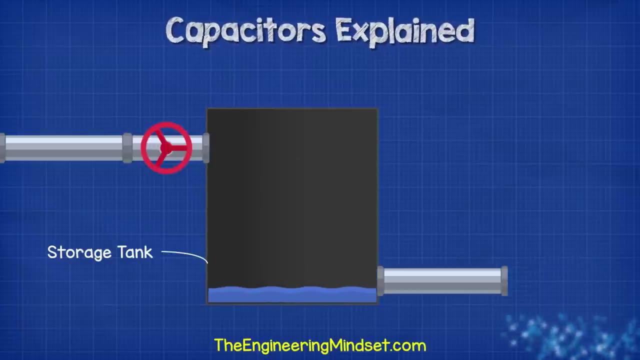 into a tank. then the tank will store some of the water, but we will continue to get water flowing out of the pipe. Now, when we close the valve, water will stop pouring into the tank, but we still get a steady supply of water out until the tank empties. Once the tank 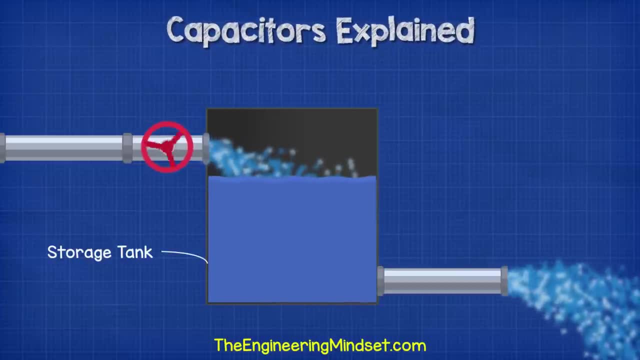 is filled again, we can open and close the valve as many times as we like. As long as we do not completely empty the tank, we will get an uninterrupted supply of water out of the end of the pipe. So we can use a water tank to store water and smooth out interruptions to the supply. 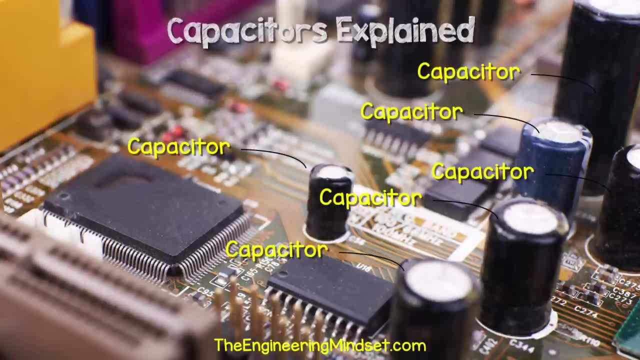 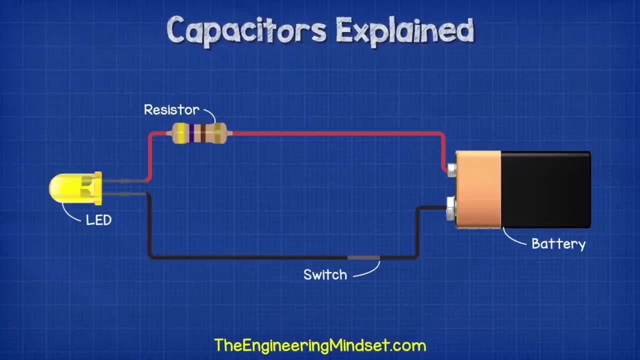 In electrical circuits the capacitor acts as the water tank and stores energy. It can release this to smooth out interruptions to the supply. If we turned a simple circuit on and off very fast without a capacitor, then the light will flash. But if we connect, 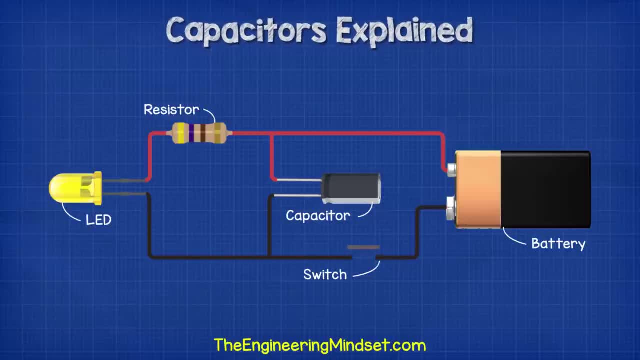 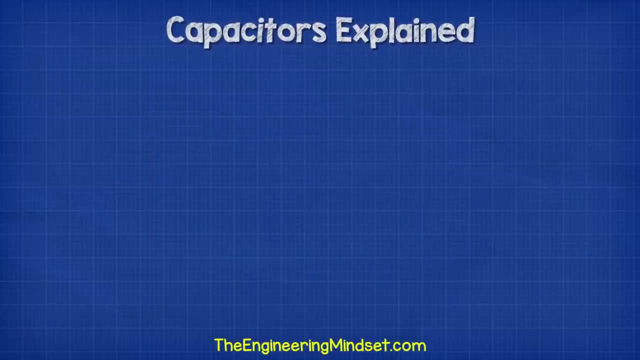 a capacitor into the circuit, then the light will remain on during the interruptions, at least for a short duration, because the capacitor is now discharging and powering the water. In a basic capacitor we have two conductive metal plates, which are typically made from. 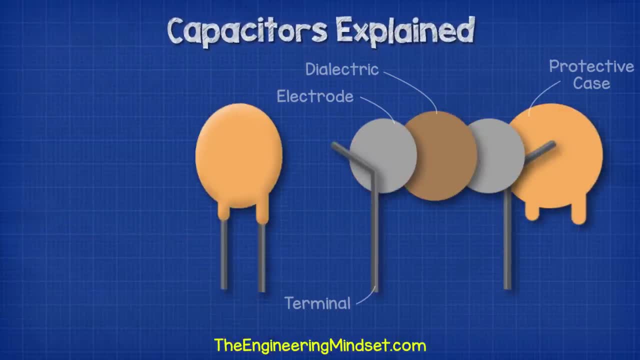 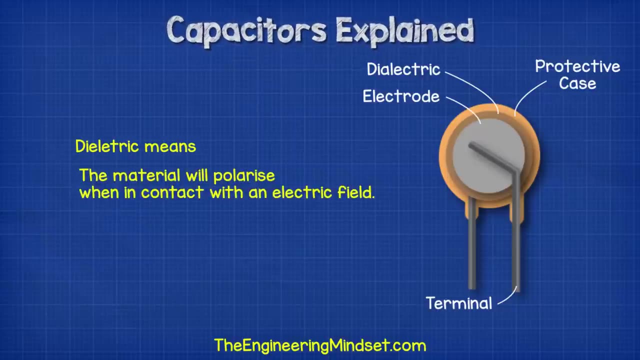 aluminium or aluminium, and these will be separated by a dielectric insulating material such as ceramic. Dielectric means the material will polarise when in contact with an electric field, and we'll see what that means shortly. One side of the capacitor is connected to. 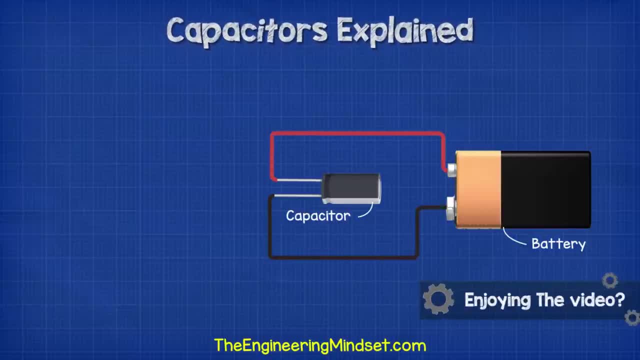 the positive side of the circuit and the other side is connected to the negative. On the side of the capacitor you will see a stripe and a symbol. This will indicate which side is the negative. If we were to connect a capacitor to a battery, the voltage will push the electrons from the 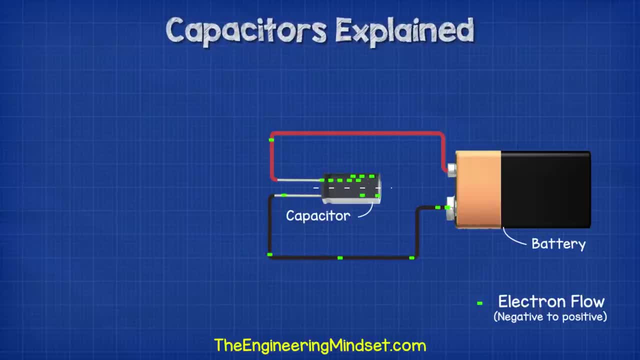 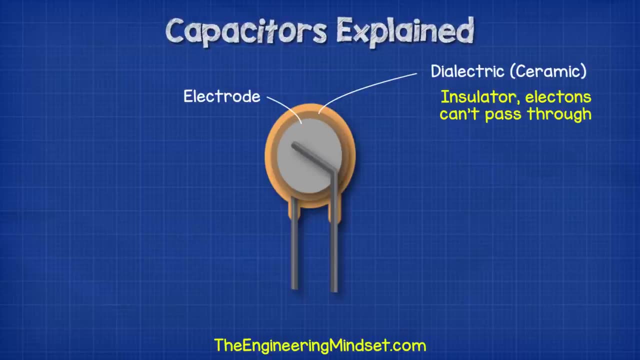 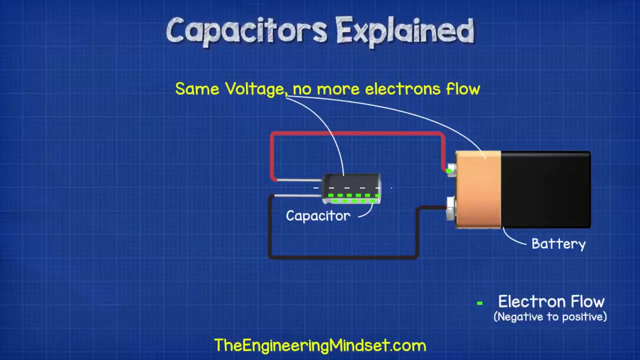 negative terminal over to the capacitor. The electrons will build up on one plate of the capacitor, while the other plate in turn releases some electrons. The electrons can't pass through the capacitor because of the insulating material. Eventually, the capacitor is the same voltage as the battery and no more electrons will flow. 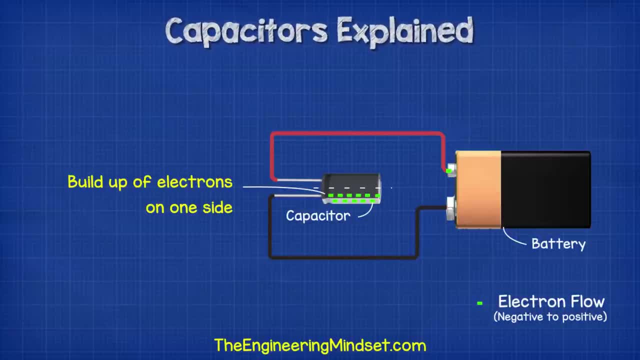 There is now a build up of electrons on one side. This means we have stored energy and we can release this when charged, Because there are more electrons on one side compared to the other and electrons are negatively charged. this means we have one side which is negative and one side which is positive. 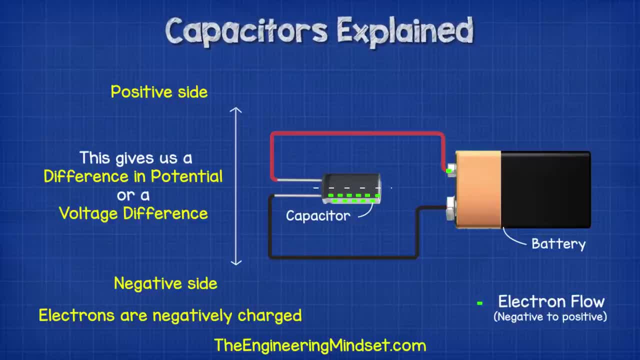 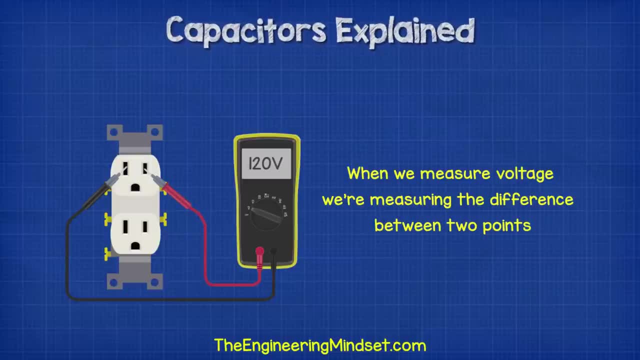 so there is a difference in potential or a voltage difference between the two and we can measure this with a multimeter. Voltage is like pressure. When we measure pressure, we're measuring the difference or potential difference between two points. If you imagine a pressurised water pipe, we 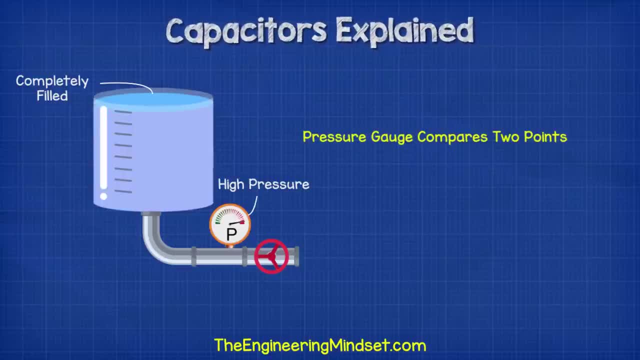 can see the pressure using a pressure gauge. The pressure gauge is compared to the voltage of the capacitor. The pressure gauge is compared to the voltage of the capacitor. The pressure point is also compared to the pressure inside the pipe's- eigentlich pressure compared to the atmospheric pressure outside the pipe. When the tank's empty, the gauge reads zero. 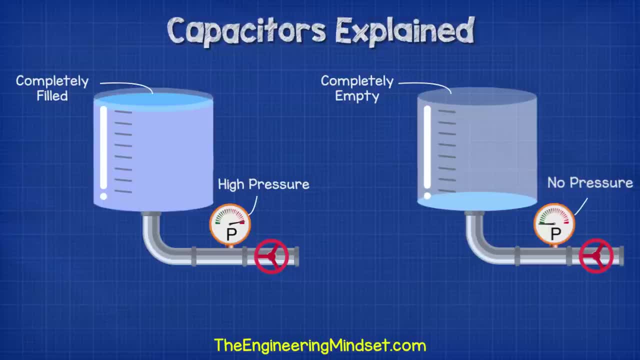 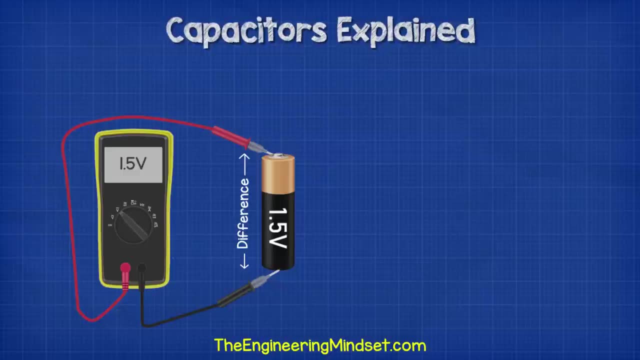 because pressure is equal to the pressure outside the tank. so the pressure gauge has nothing to compare against. both are the same pressure, The same. with voltage. We're comparing the difference between two points. If we measure across a 1.5-volt battery, then we read a difference of 1.5-volts between each end. 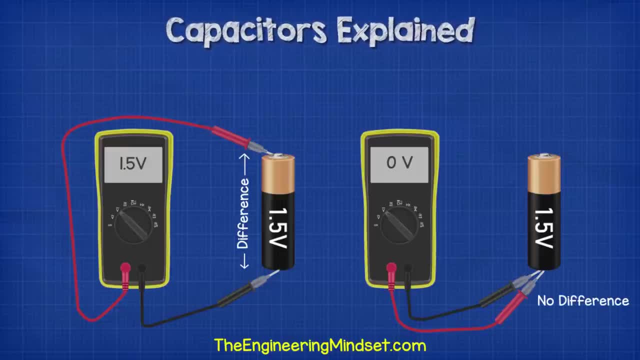 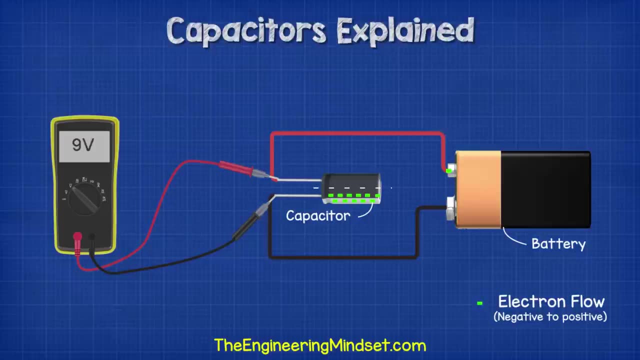 Thank you, But if we measure the same end, then we read zero because there's no difference and it's going to be the same. Coming back to the capacitor, we measure across and read a voltage difference between the two because of the build up of electrons. 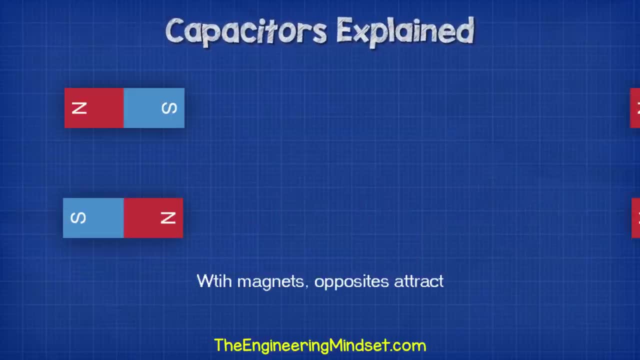 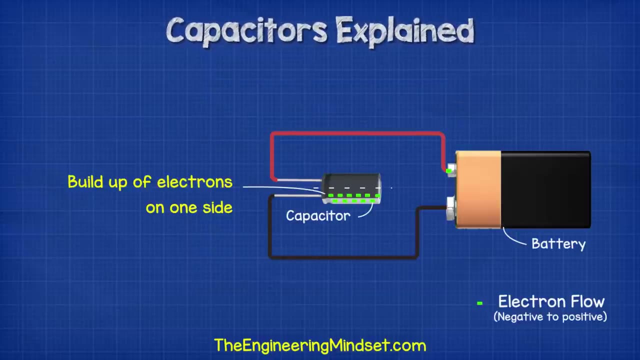 We still get this reading, even when we disconnect the battery. If you remember, with magnets, opposites attract and pull towards each other. The same occurs with the build up of negatively charged electrons: They are attracted to the positively charged particles of their atoms on the opposite plate. 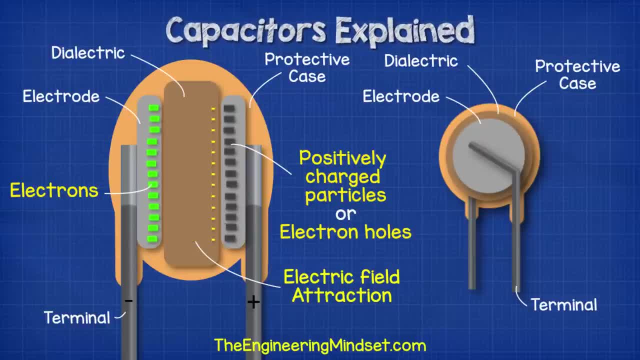 But they can never reach each other because of the insulating material. This pull between the two sides is an electric field which holds the electrons in place until another path is made. If we then place a small lamp into the circuit, a path now exists for the electrons to flow. 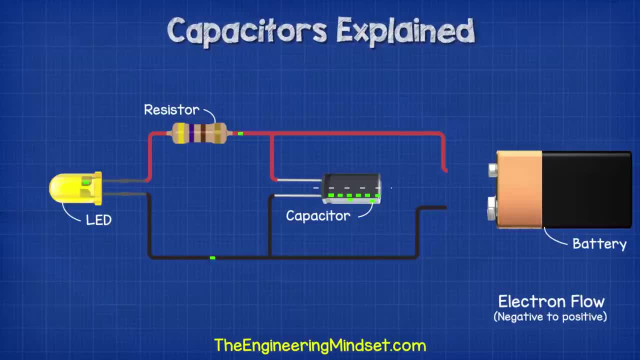 and reach the opposite side, So the electrons will flow through the lamp powering it, and the electrons will reach the other side of the capacitor. This will only last a short duration though, until the build up of electrons equalises on each side. Then the voltage is zero, so there is no pushing force and no electrons will flow. 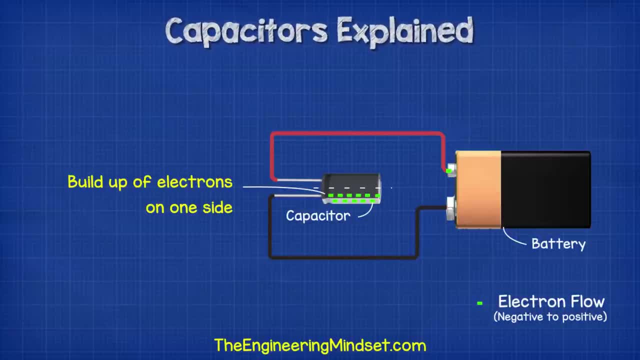 There is now a build up of electrons on one side. This means we have stored energy and we can release this when charged, Because there are more electrons on one side compared to the other and electrons are negatively charged. this means we have one side which is negative and one side which is positive. 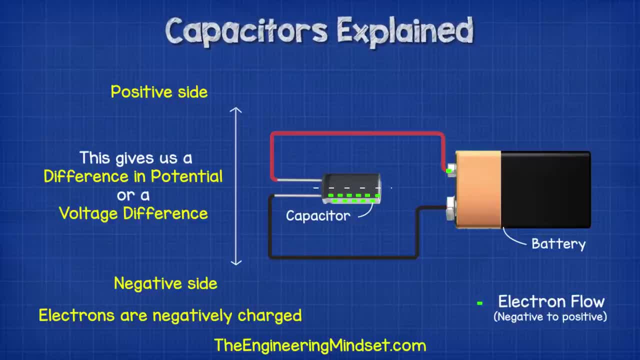 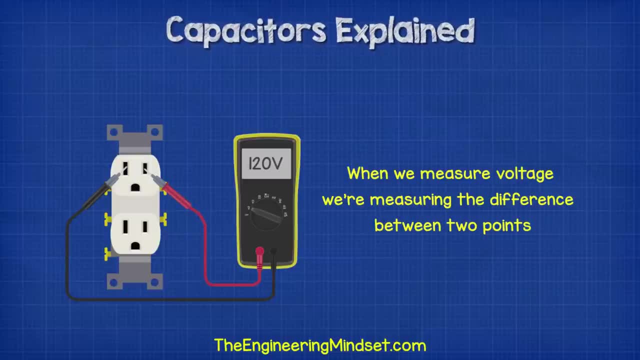 so there is a difference in potential or a voltage difference between the two and we can measure this with a multimeter. Voltage is like pressure. When we measure pressure, we're measuring the difference or potential difference between two points. If you imagine a pressurised water pipe, we 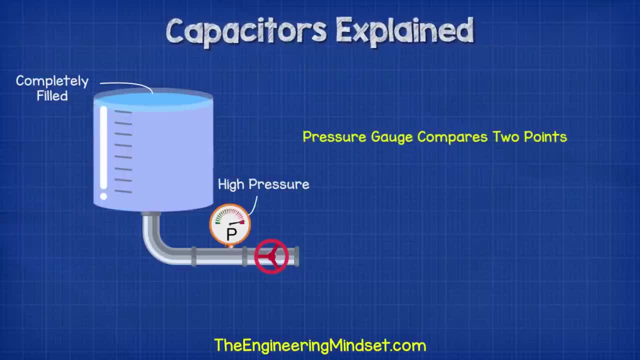 can see the pressure using a pressure gauge. The pressure gauge is compared to the voltage of a battery. The pressure gauge is compared to the voltage of a battery. We're comparing two different points. also: The pressure inside the pipe compared to the atmospheric pressure outside the pipe When the tank is empty. the gauge 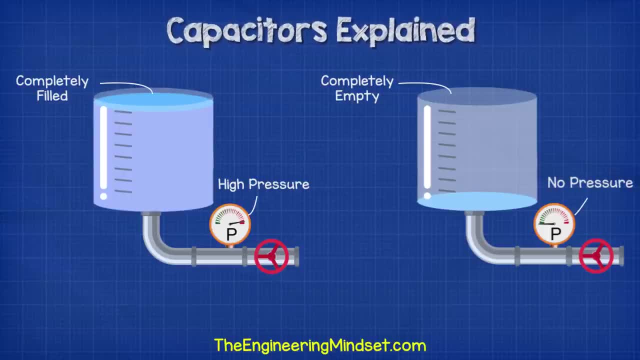 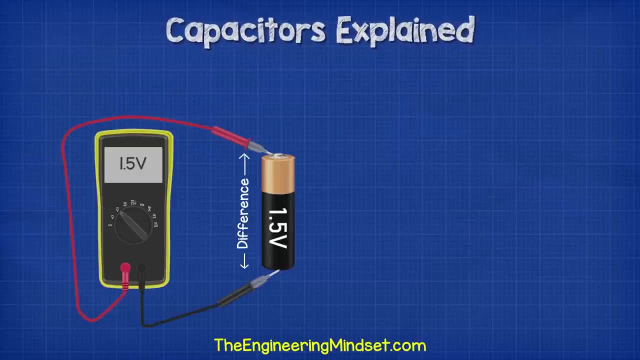 reads zero because the pressure inside the tank is now equal to the pressure outside the tank, so the gauge has nothing to compare against. Both are the same pressure, The same. with voltage. We're comparing the difference between two points. If we measure across a 1.5V battery, then we read a difference of 1.5V between each end. 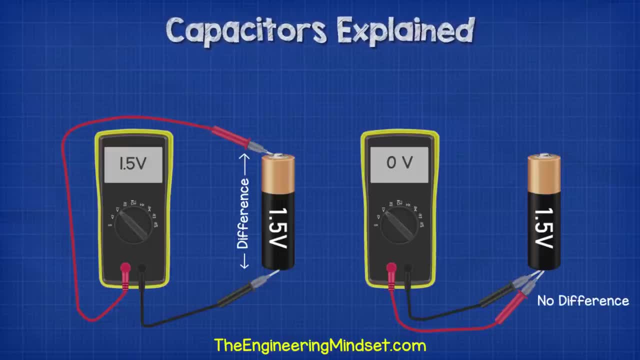 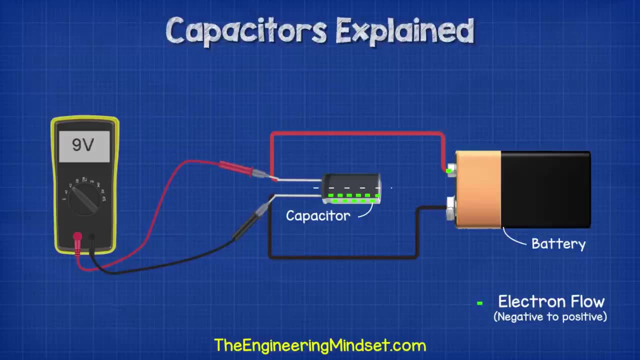 But if we measure the same end, then we read zero because there's no difference and it's going to be the same. Coming back to the capacitor, we measure across and read a voltage difference between the two because of the buildup of electrons. We still get this reading, even when we disconnect. 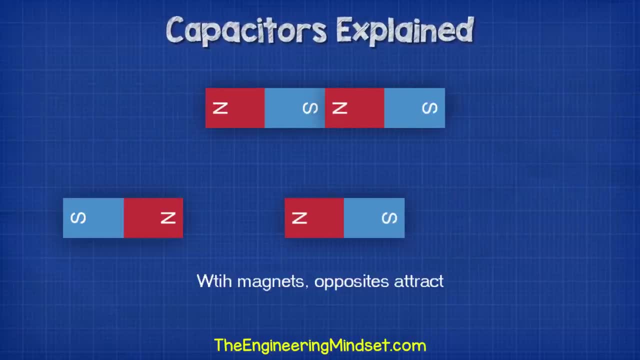 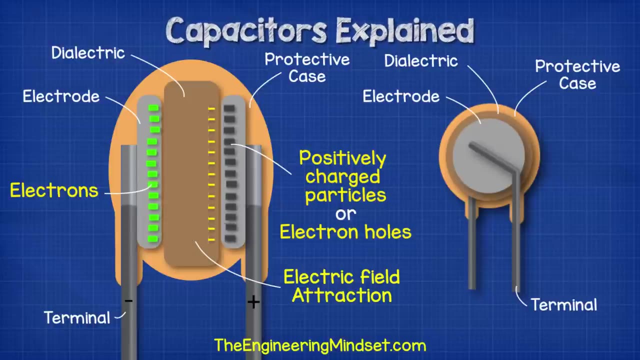 the battery. If you remember, with magnets, opposites attract and pull towards each other. The same occurs with the buildup of negatively charged electrons. They are attracted to the positively charged particles of their atoms on the opposite plate, But they can never reach each other because of the insulating material. 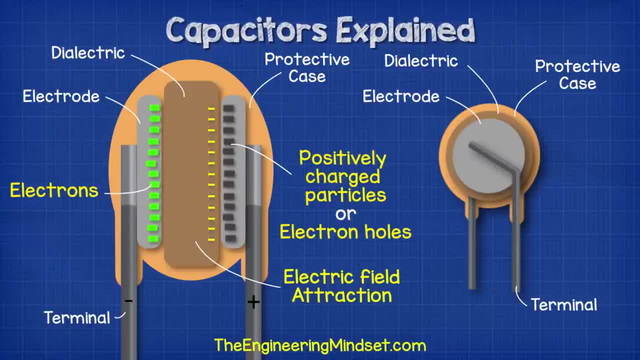 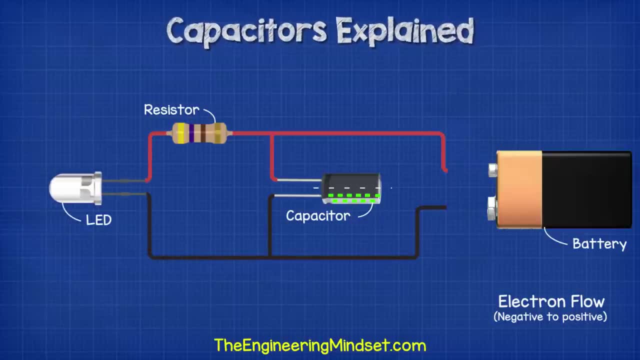 This pull between the two sides is an electric field which holds the electrons in place until another path is made. If we then place a small lamp into the circuit, a path now exists for the electrons to flow and reach the opposite side, So the electrons will flow. 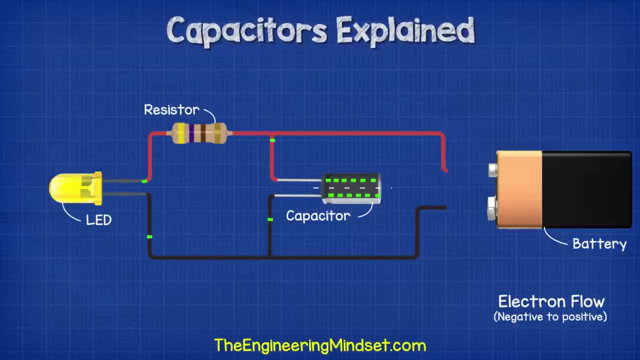 through the lamp powering it, and the electrons will reach the other side of the capacitor. This will only last a short duration, though, until the buildup of electrons equalises on each side. Then the voltage is zero, So there is no pushing force and no electrons will flow. 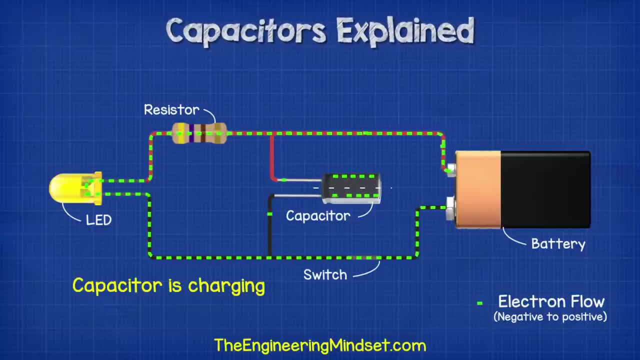 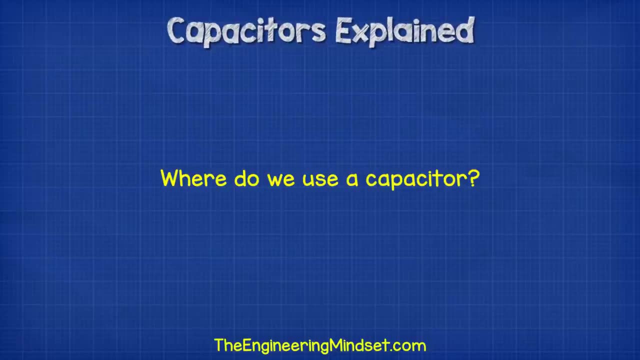 Once we connect the battery again, the capacitor will begin to charge. This allows us to interrupt the power supply, and the capacitor will provide power during these interruptions. So where do we use capacitors? They look a little bit different, but they're easy to spot. 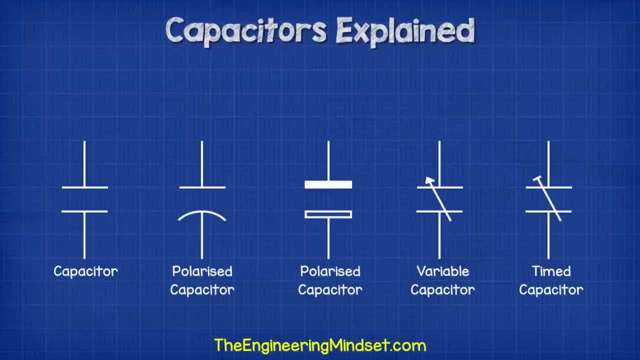 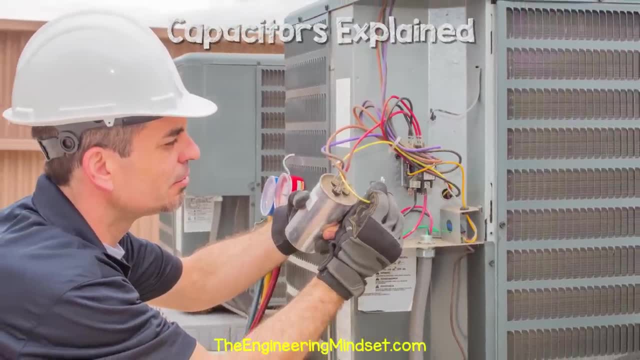 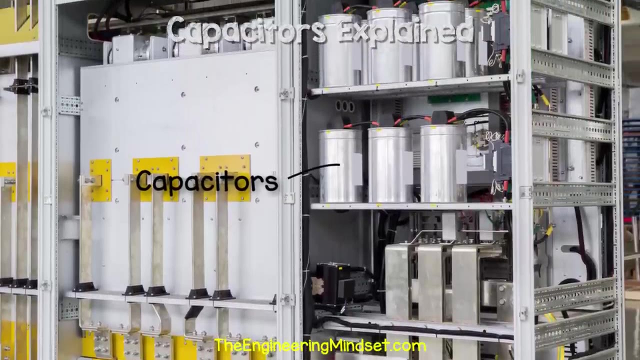 In circuit boards. they tend to look something like this And we see them represented in engineering drawings with symbols like these. We can also get larger capacitors, which are used, for example, on induction motors. This is a very common problem. We can get even larger ones, which are used to create poor power factor in large buildings. 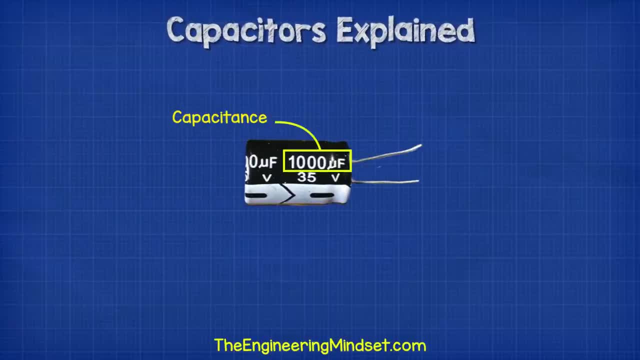 On the side of the capacitor we will find two values. These are the capacitance and the voltage. We measure capacitance of the capacitor in the unit of farads, which we show with a capital F, although we will usually measure a capacitor in microfarads. 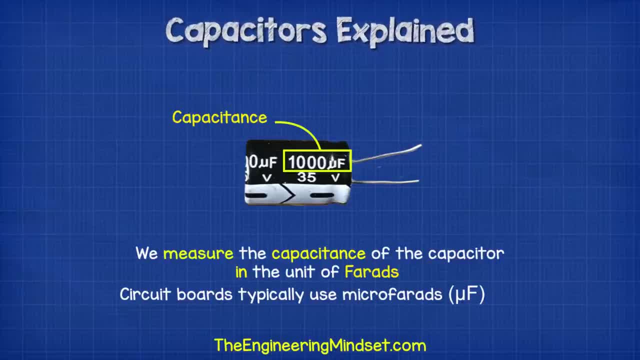 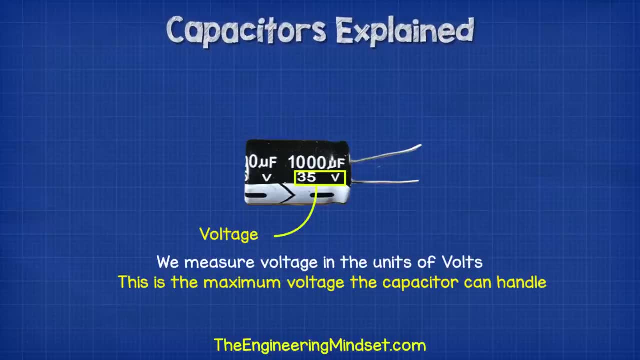 With microfarads. we just have a symbol before this which looks something like a letter U with a tail. The other value is our voltage, which we measure in volts with a capital F. We measure the voltage in volts with a capital F On the capacitor. the voltage value is the maximum voltage which the capacitor can handle. 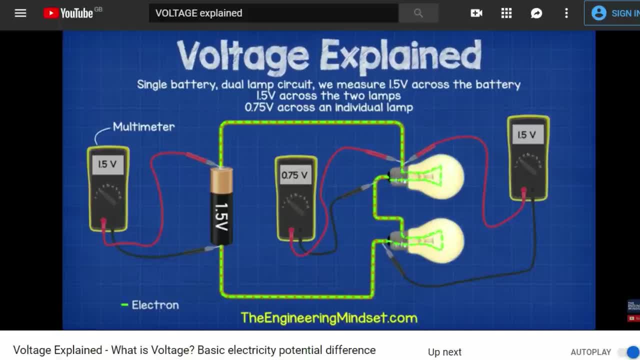 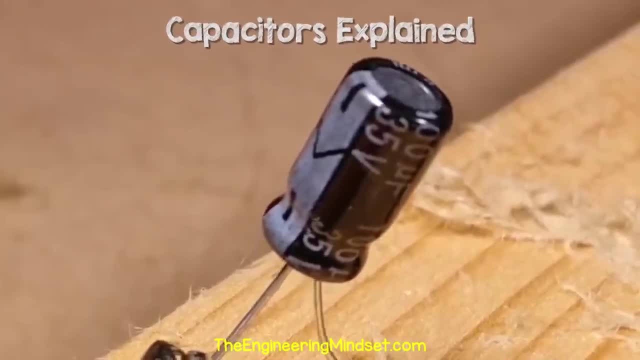 We've covered voltage in detail in a separate video. do check that out. link's down below. As I said, the capacitor is rated to handle a certain voltage. If we were to exceed this then the capacitor will explode. Let's have a look at that in slow motion. 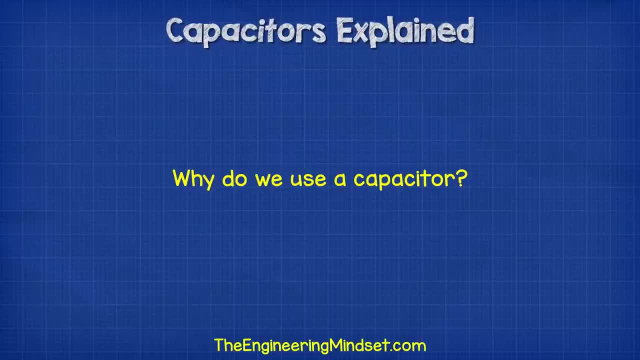 Pretty cool. So why do we use capacitors? One of the most common applications of capacitors in large buildings is the use of capacitors in large buildings. Capacitors in large buildings are used to generate current. Capacitors in large buildings are used to generate current. 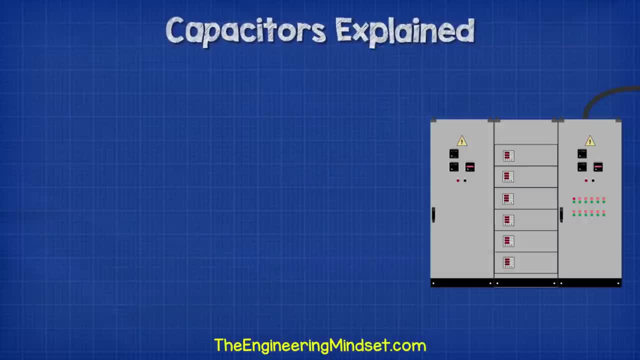 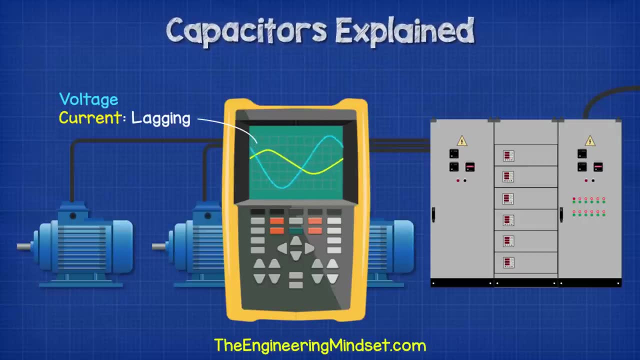 When too many inductive loads are placed into a circuit, the current and the voltage waveforms will fall out of sync with each other, and the current will lag behind the voltage. We then use capacitor banks to counteract this and bring the two back into alignment. 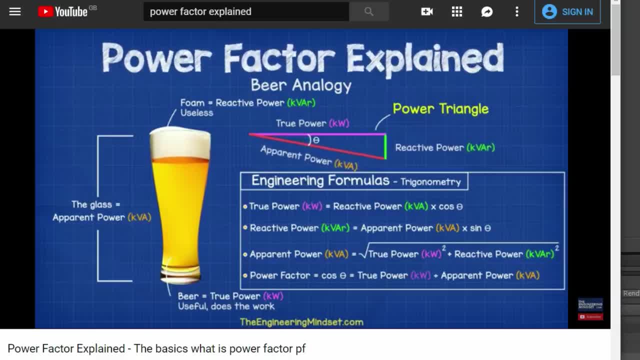 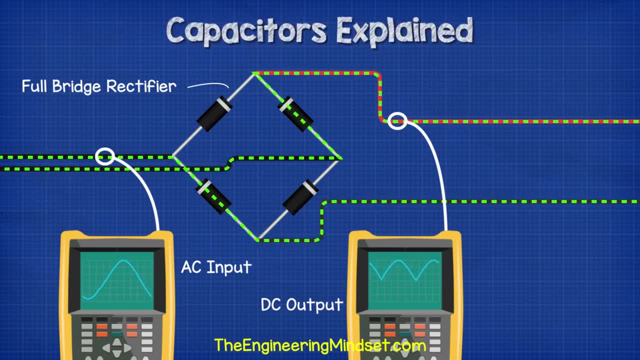 We've covered power factor before in great detail. do check that out. link's down below. Another very common application is to smooth out peaks when converting AC to DC power. When we use a full bridge rectifier, the AC sine wave is the same as the AC sine wave. 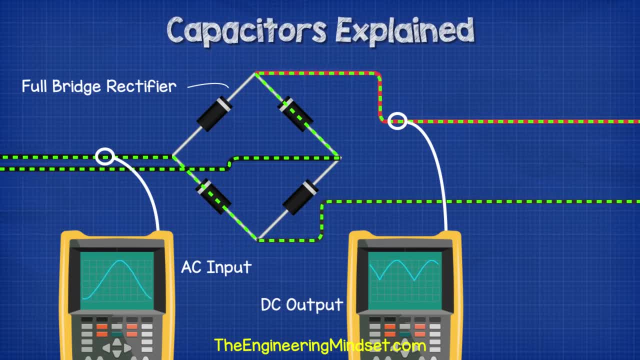 When we use a full bridge rectifier, the AC sine wave is the same as the DC power. The DC sine wave is flipped to make the negative cycle flow in a positive direction. The DC sine wave is flipped to make the negative cycle flow in a positive direction. 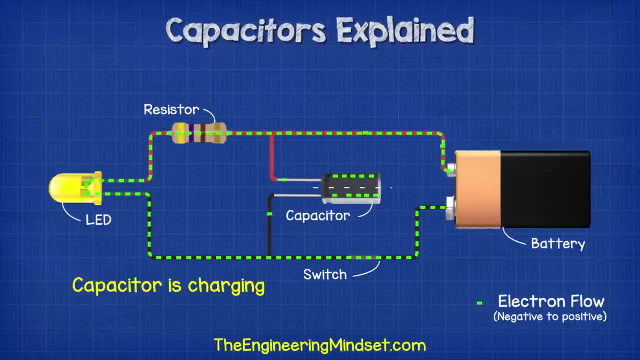 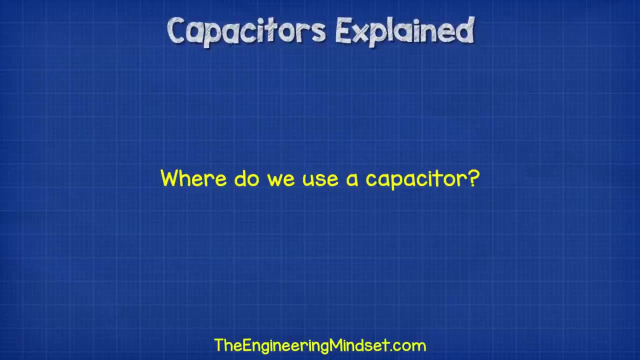 Once we connect the battery again, the capacitor will begin to charge. This allows us to interrupt the power supply and the capacitor will provide power during these interruptions. So where do we use capacitors? They look a little bit different, but they're easy to spot In circuit boards. they tend. 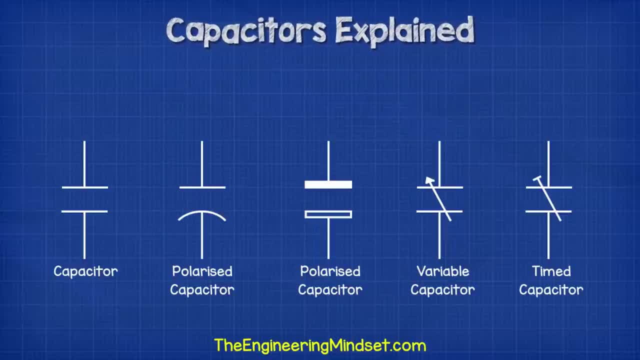 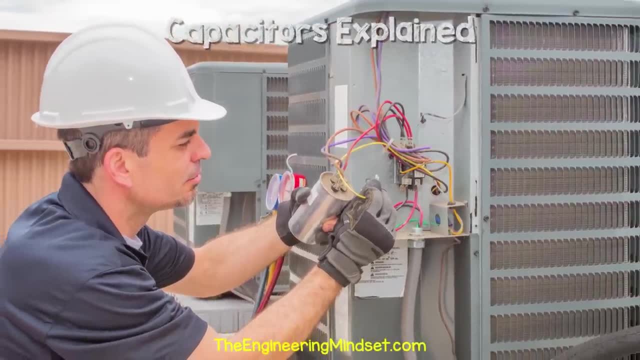 to look something like this, And we see them represented in engineering drawings with symbols like these. We can also get larger capacitors, which are used, for example, on induction motors, ceiling fans and air conditioning units. We can get even larger ones, which are used 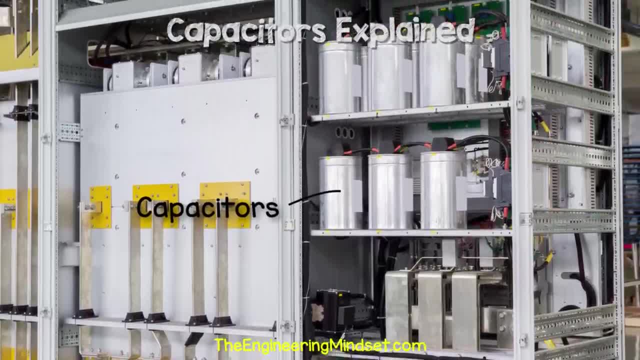 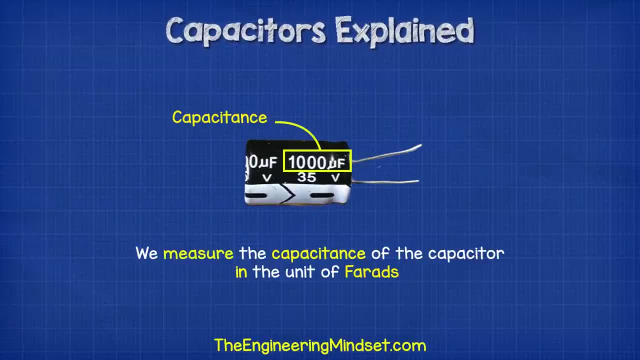 to create poor power factor in large buildings. On the side of the capacitor we will find two values. These are the capacitance and the voltage. We measure capacitance of the capacitor in the unit of farads, which we show with a capital F, although we will usually measure a capacitor in microfarads With microfarads. 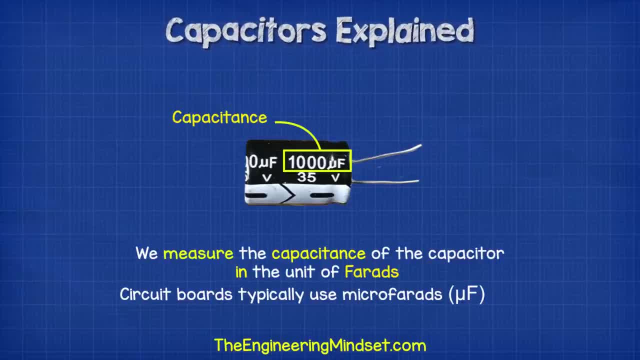 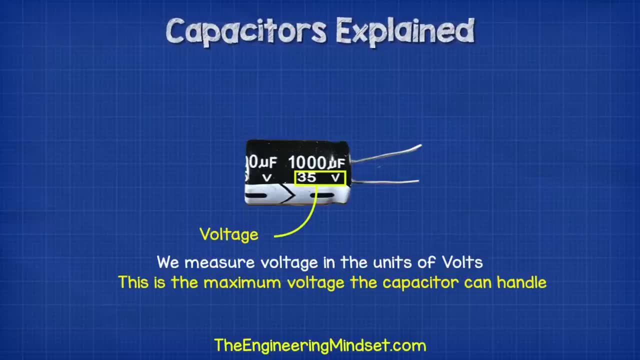 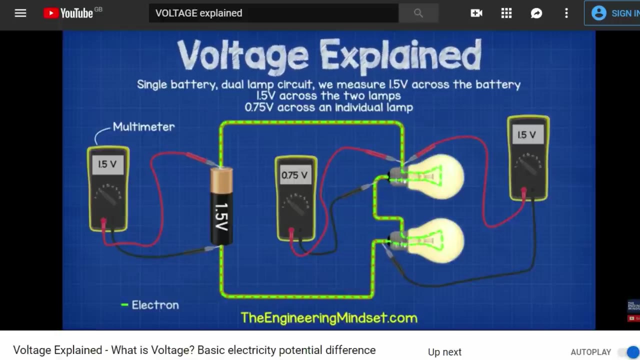 we just have a symbol before this which looks something like a letter U with a tail. The other value is our voltage, which we measure in volts with a capital V On the capacitor. the voltage value is the maximum voltage which the capacitor can handle. We've covered voltage in detail in a separate video. do check that out. link's down below. 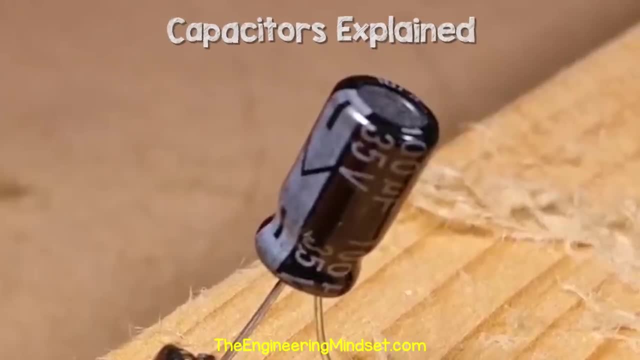 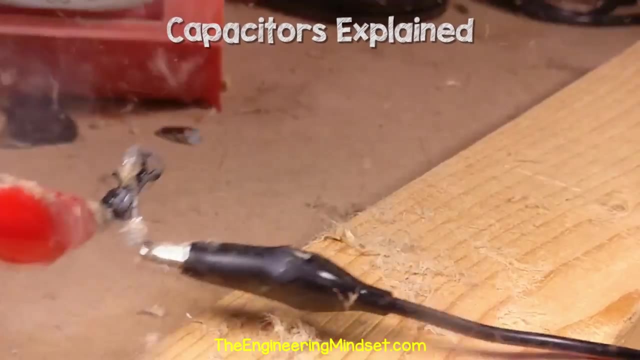 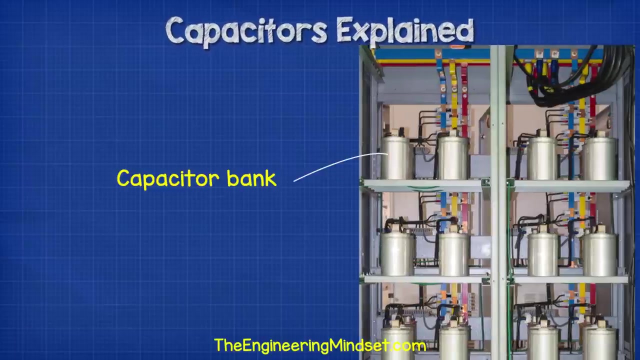 As I said, the capacitor is rated to handle a certain voltage. If we were to exceed this, then the capacitor will explode. Let's have a look at that in slow motion- Pretty cool. So why do we use capacitors? One of the most common applications of capacitors in large 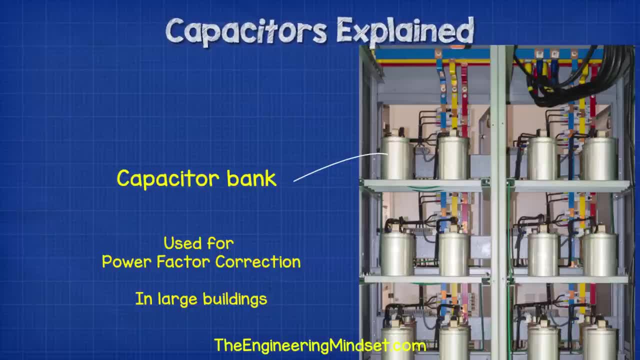 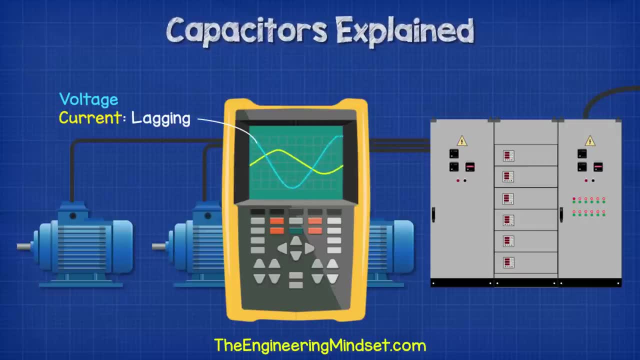 buildings is for power factor. When too many inductive loads are placed into a circuit, the current and the voltage waveforms will fall out of sync with each other and the current will lag behind the voltage. We then use capacitor banks to counteract this and bring the two back into alignment. 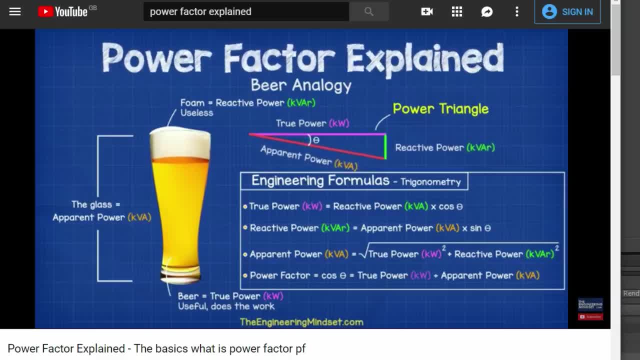 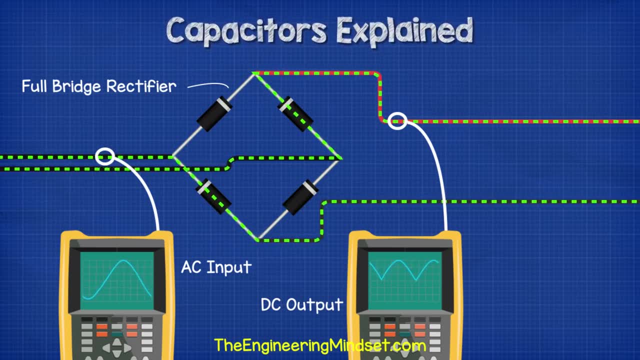 We've covered power factor before in great detail. do check that out. link's down below. Another very common application is to smooth out peaks when converting AC to DC power. When we use a full bridge rectifier, the AC sine wave is flipped to make the negative. 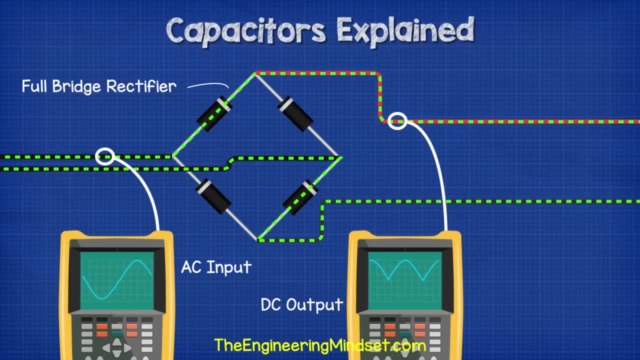 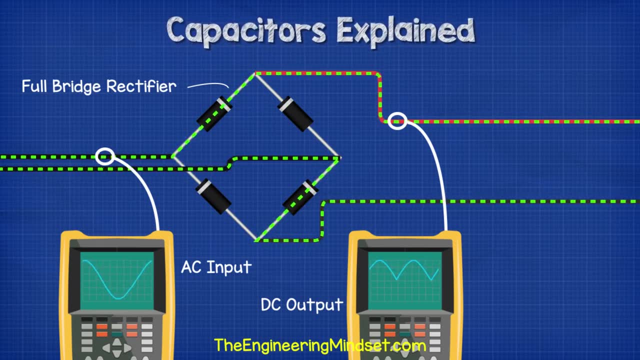 cycle flow in a positive direction. This will trick the circuit into thinking it's getting direct current. but one of the problems with this method is the gaps in between the peaks. But, as we saw earlier, we can use a capacitor to release energy into the circuit during.